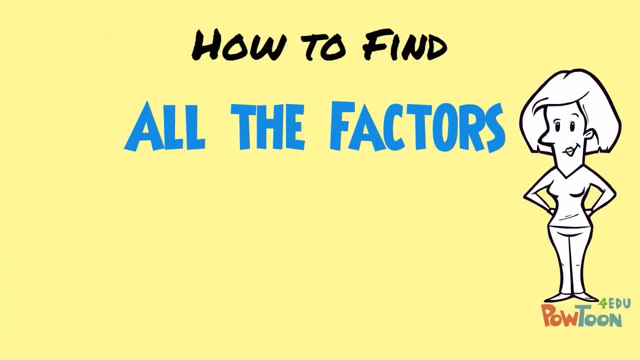 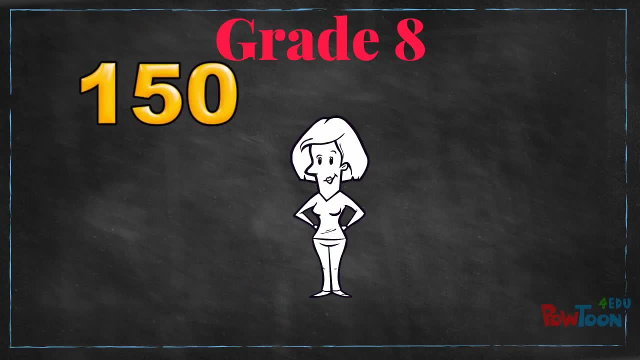 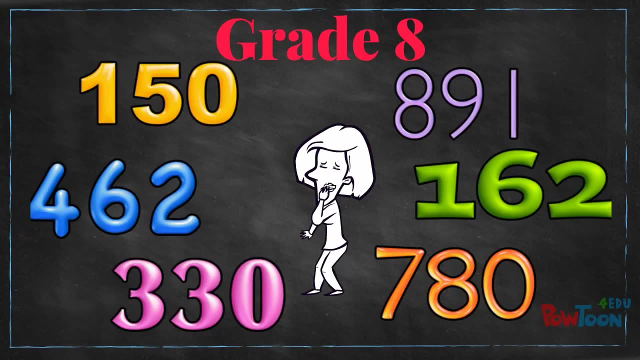 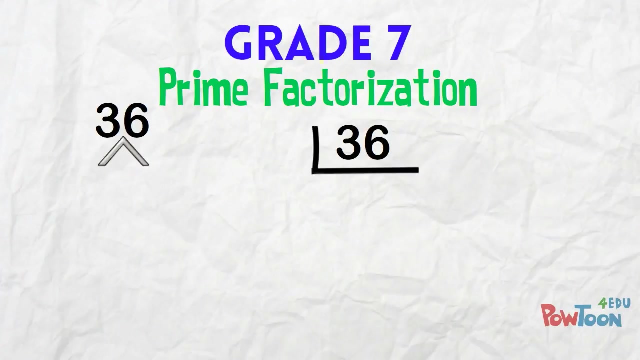 How to find ALL THE FACTORS of ANY NUMBER FAST. If you remember what to do- and this is familiar to you- That's GREAT. You're nearly there ALREADY. If you're not sure about prime factorization or you want to review it, 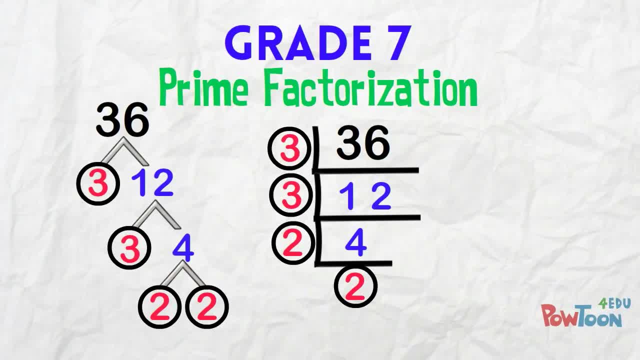 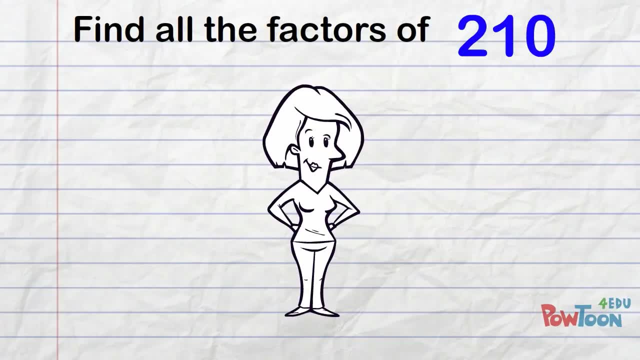 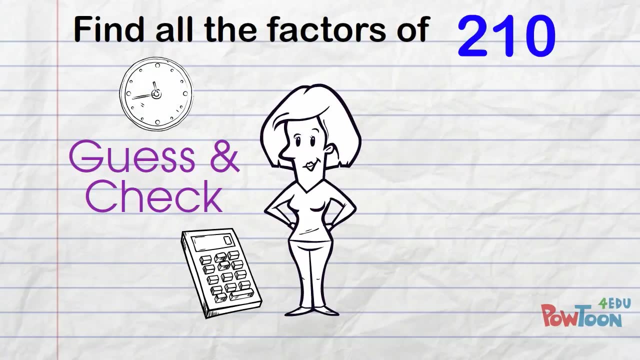 check out these films first, then come back for this video. OK, we are going to find ALL THE FACTORS of. We could try a guess and check approach and use a calculator to find all the factors. To be honest, this will take us. 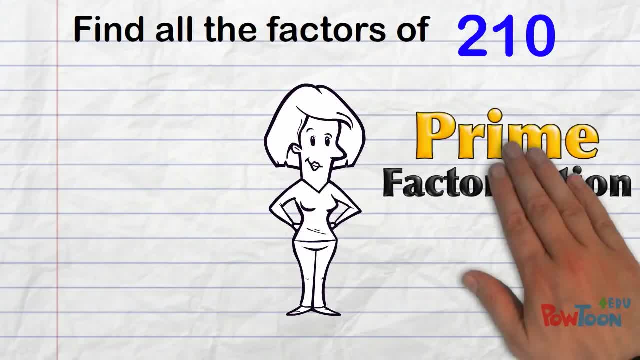 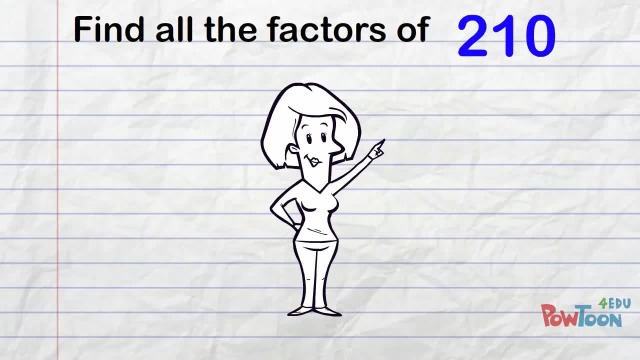 ages. Instead we go straight to PRIME FACTORIZATION. to make life easy, 210 is NOT in any multiplication table we know, So we can start the prime factorization with DIVISION. Our number is even, so we start with 2.. 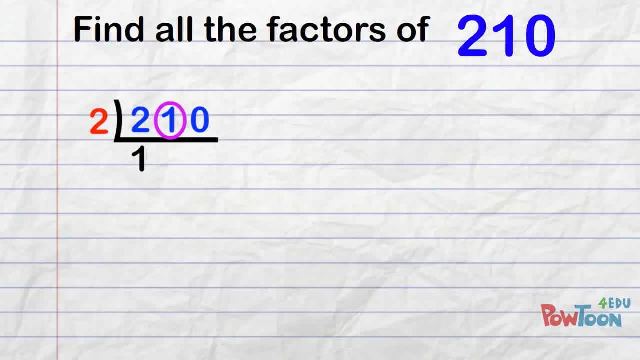 2 x 2? 1, 2 x 1? 0, 2 x 10? 5 x 2? 10, 105. Now of course we divide by 5.. 5 x 10? 2, 5 x 5? 1. 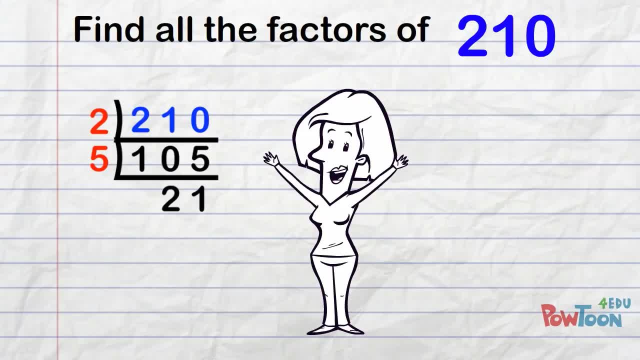 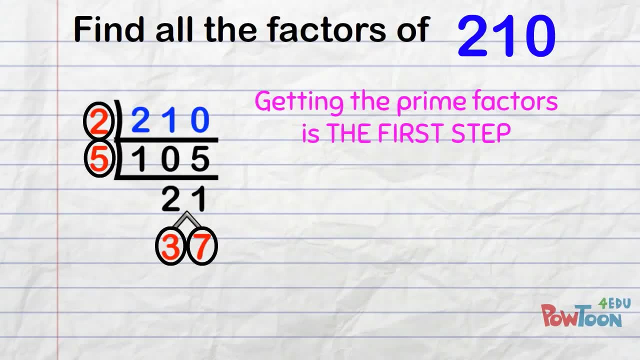 21 GREAT. You get 21 from 3 x 7. They're both prime. We circle all the primes. Getting the prime factors is our first step. Already you can see here we've found some of the factors of 210.. 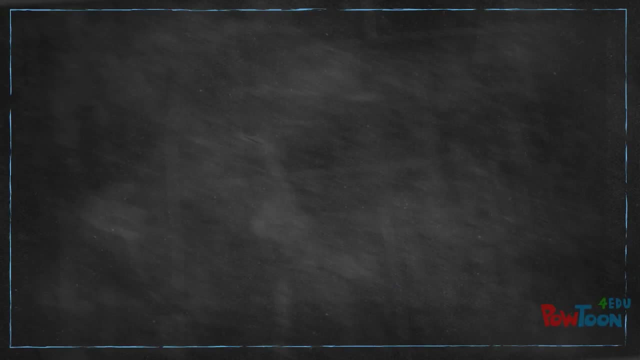 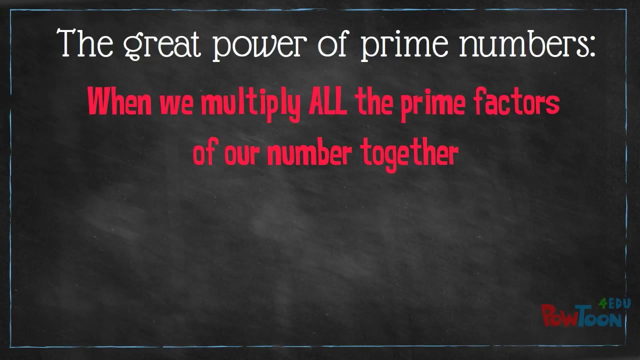 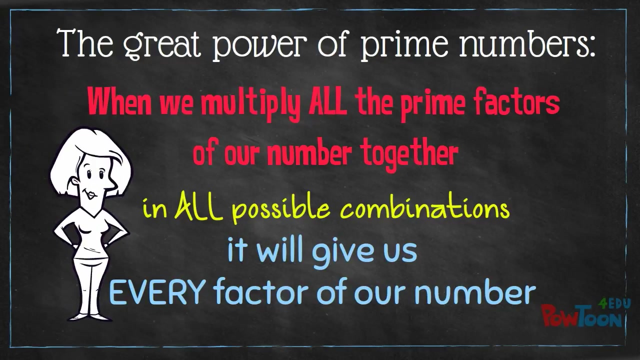 But there are still more to find. And here's the great power of prime numbers. When we multiply all the prime factors of our number together in all possible combinations, it will give us every factor of our number, 210 in this case. 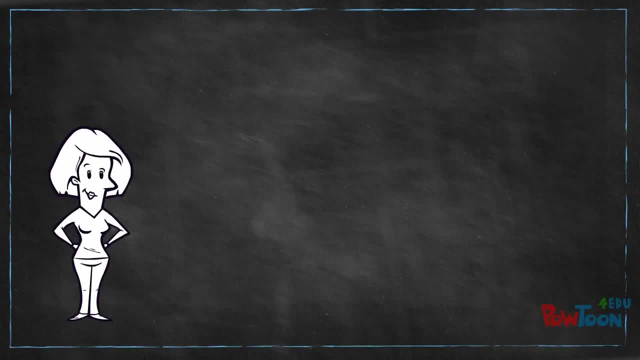 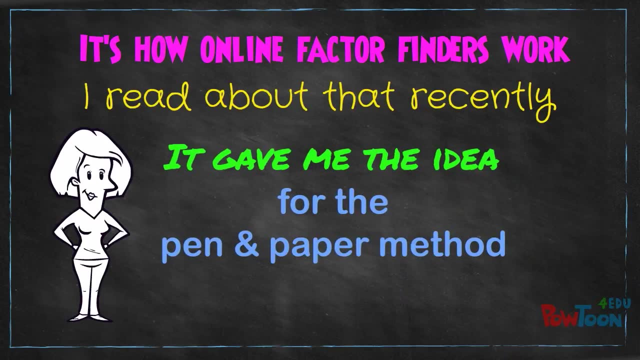 That's such a powerful tool And it's how online factor finders work. I read about that recently, and it gave me the idea for the pen and paper method that I'm going to show you in a moment. It works every time. 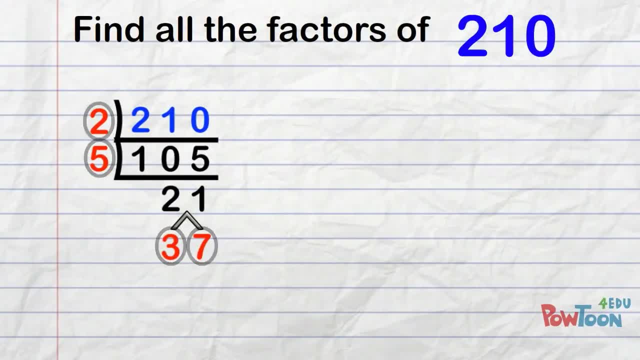 and I want to share it with you. First we need a sensible working area. We list our primes clearly, spaced out nicely, and then we multiply On the first line. we multiply by our first number. So 2 x 3 is 6.. 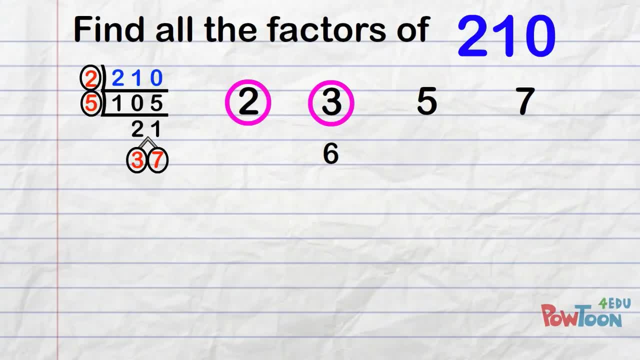 The 6 came from 2 x 3, so put it under the 3.. 2 x 5 is 10 and 2 x 7 is 14.. Next line: 3 x everything. 3 x 2. we've already got. 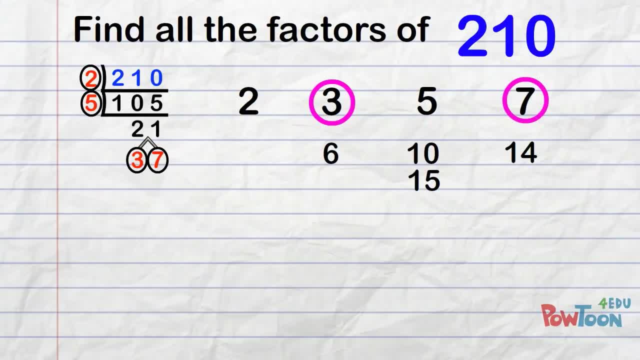 3 x 5 is 15.. And 3 x 7 is 21.. Next line: 5.. 5 x 2 is done, 5 x 3 is done. 5 x 7 is 35.. I don't need a line for 7. 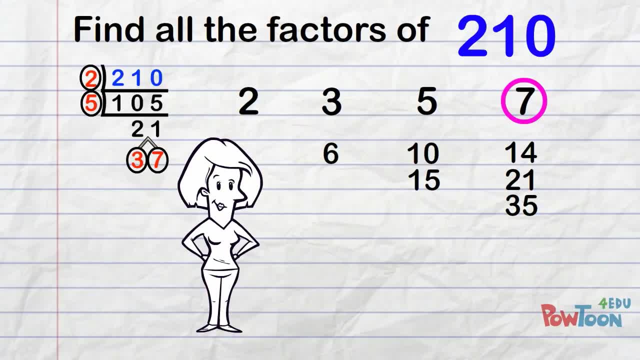 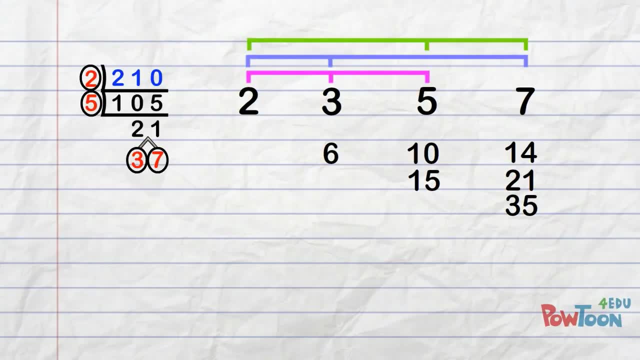 because 7 has already been multiplied by 2, 3 and 5.. We do also have to multiply combinations of our prime factors together too. 2 x 3 x 5 is the same as 6 x 5. That's 30.. 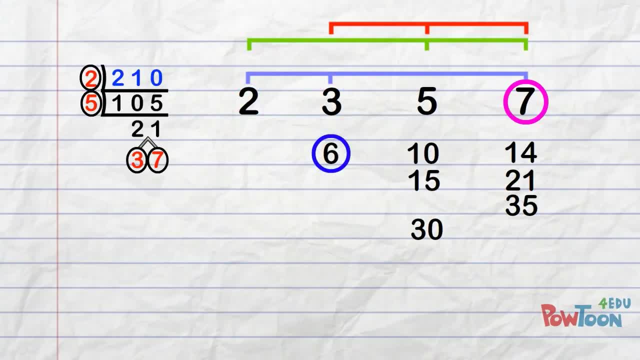 2 x 3 x 7 is the same as 6 x 7.. 42.. 2 x 5 x 7 is the same as 10 x 7.. 70.. 3 x 5 x 7 is the same as 15 x 7.. 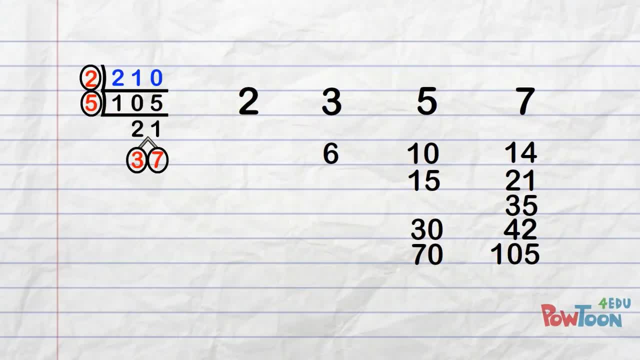 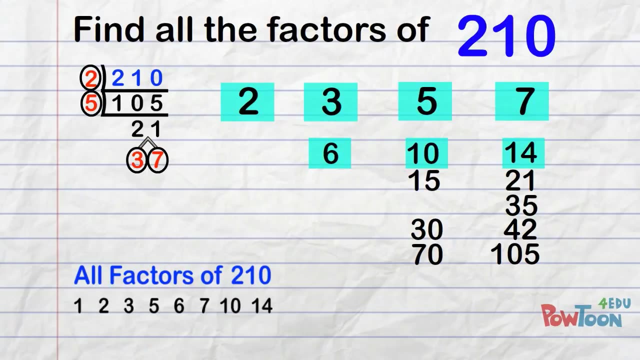 That's 105.. To finish off, we list all the factors of 210 in ascending order. Start with 1, then 2, 3, 5, 6, 7, 10, 14, 15. Just do what I'm doing. go through your list. 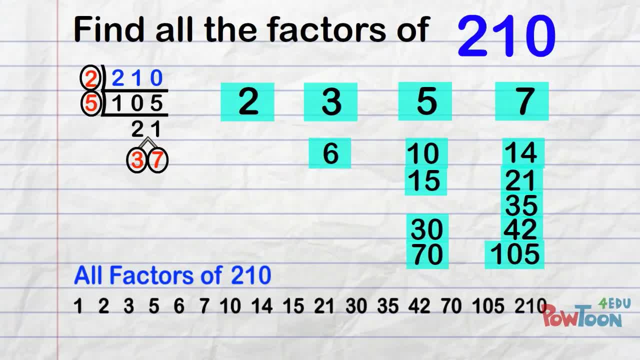 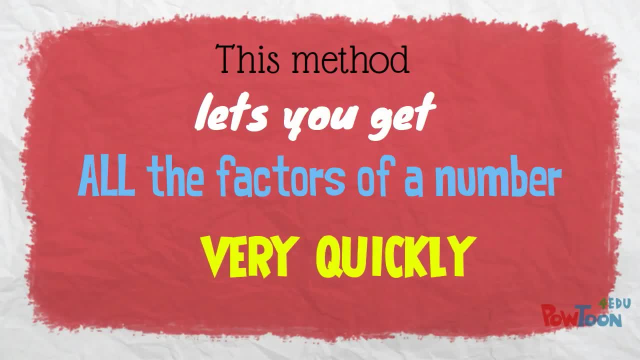 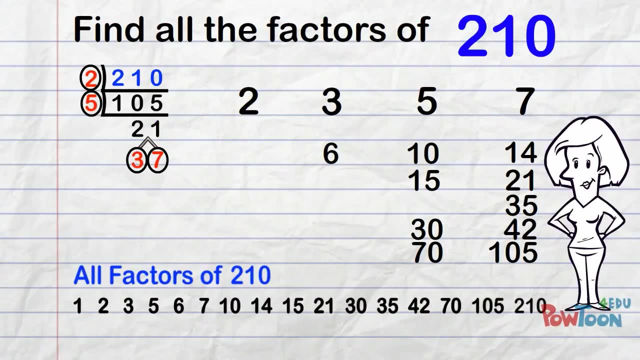 and when they're all done, you finish up with 210, the number itself. This method lets you get at all the factors of a number very quickly- Way faster than guess and check with a calculator. When you use this method, set your work out like I did here.